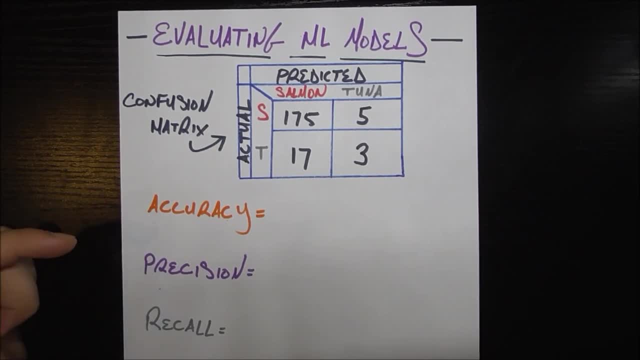 Well, that is one possible metric you can use, and it's called accuracy. But we'll see why that's not always the best metric you want to use, or at least it's not the only metric you want to calculate, to see how good of a job you've done. So we're going to be using the same type of 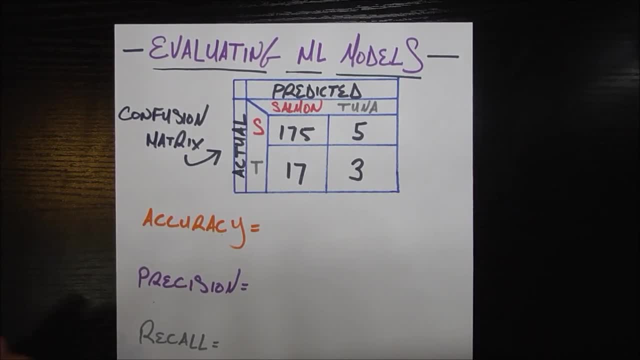 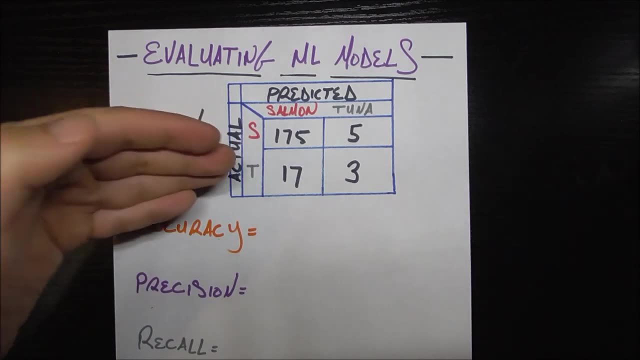 framework we've used in previous videos about we're trying to classify some mystery fish as either a salmon or a tuna, And let's say that we've run whatever machine learning algorithm that we want to run and these are our results. So this type of 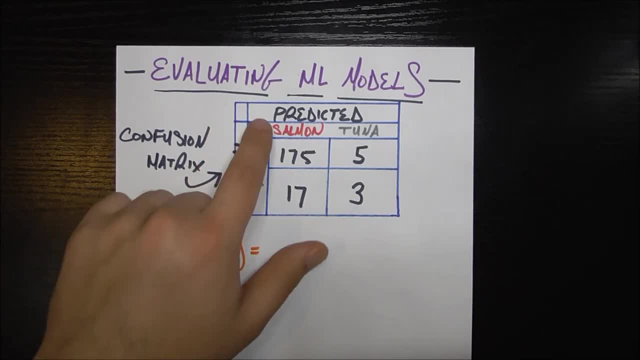 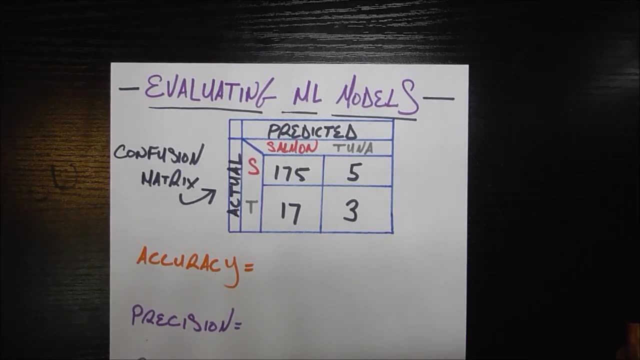 matrix that we're going to be using is called accuracy, And we're going to use this type of matrix right here, where we have our actual labels on the left and we have our predicted labels up here on the top. It's called a confusion matrix and it basically just tells us how many things 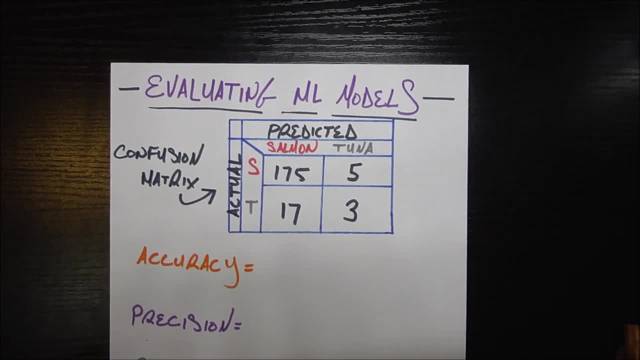 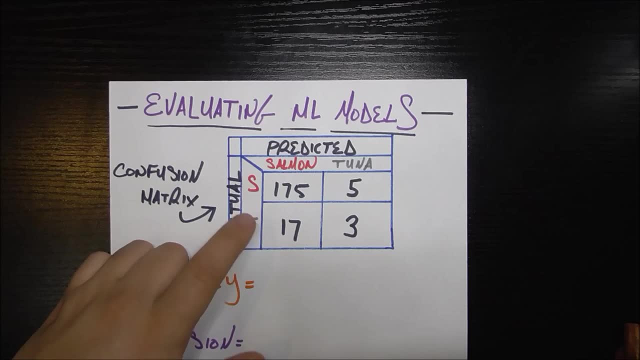 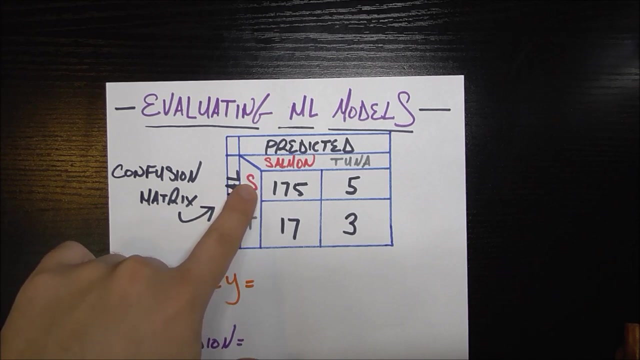 we got correct out of each category that we predicted. So let's get a little bit familiar with this matrix before looking at the different metrics we'll use. So S is salmon, T is tuna, For example, this 5 right here says that there was five cases where the mystery fish was actually a. 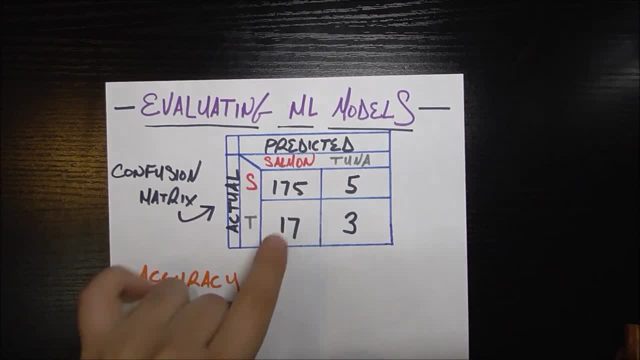 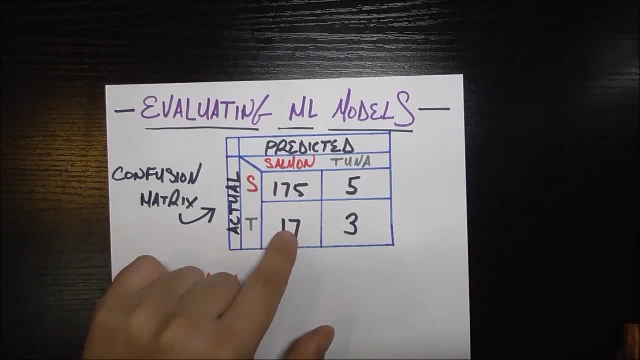 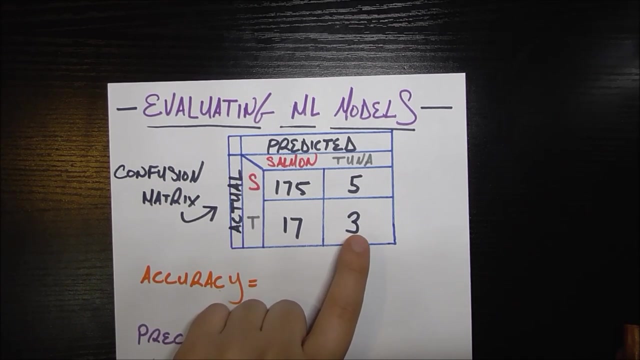 salmon, but I predicted it to be a tuna, So I was wrong here. This is also a wrong situation. It's just the other way, where the mystery fish was actually a tuna, but I predicted it to be a salmon. In opposition, we have this 3 here, which is a correct guess. We're saying here that 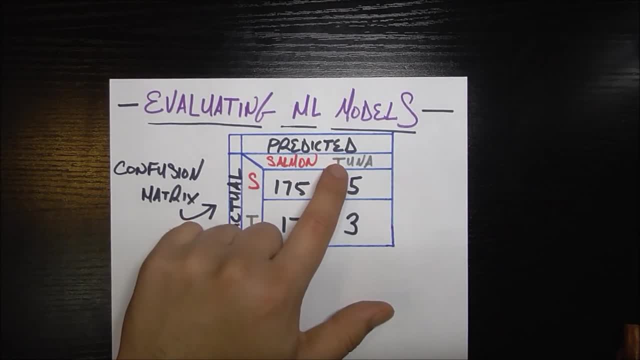 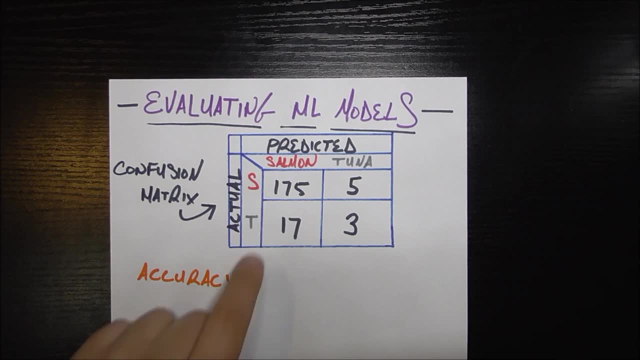 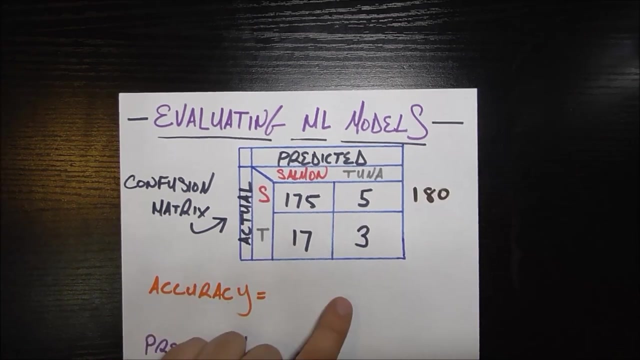 there was three cases where it was actually a tuna and we predicted it to be a tuna. So one thing to note right here is that we had many, many more salmon than tuna. So we had, it seems like 180 actual salmon and 20 actual tuna. Okay, so let's go ahead and calculate that. 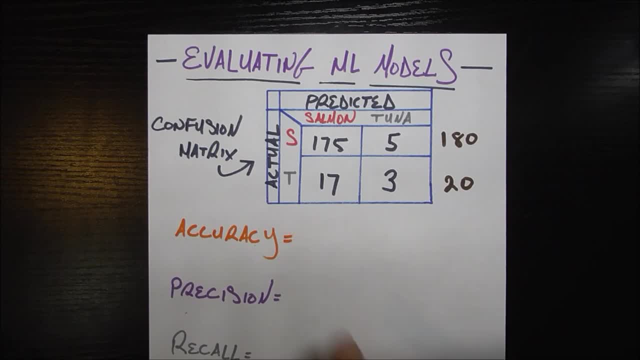 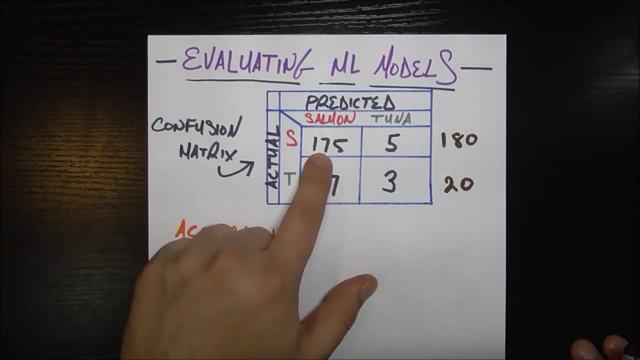 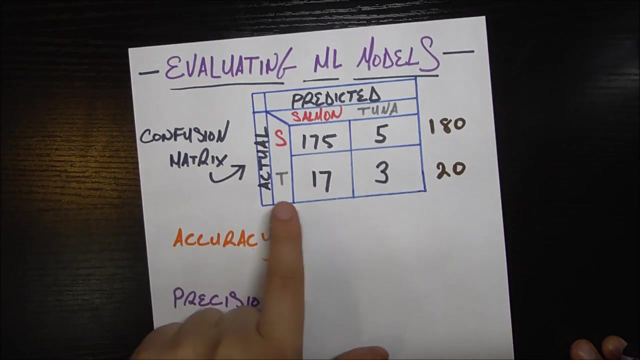 seemingly obvious accuracy metric, Right. So accuracy simply measures out of how many total guesses I made. So correct would be this 175,, which is predicting salmon, and its actually a salmon, plus this 3, predicting and it's actually a tuna. So I get 178 correct guesses Out of how many total guesses, if you. 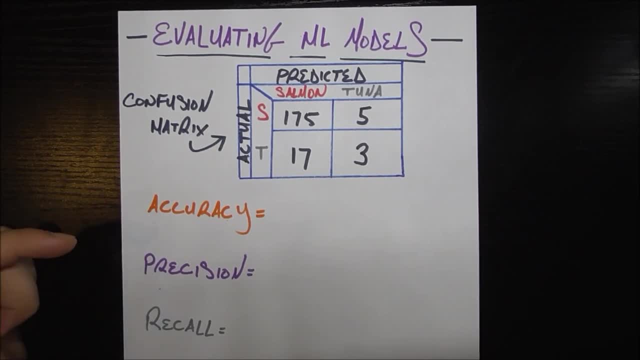 Well, that is one possible metric you can use, and it's called accuracy. But we'll see why that's not always the best metric you want to use, or at least it's not the only metric you want to calculate, to see how good of a job you've done. So we're going to be using the same type of 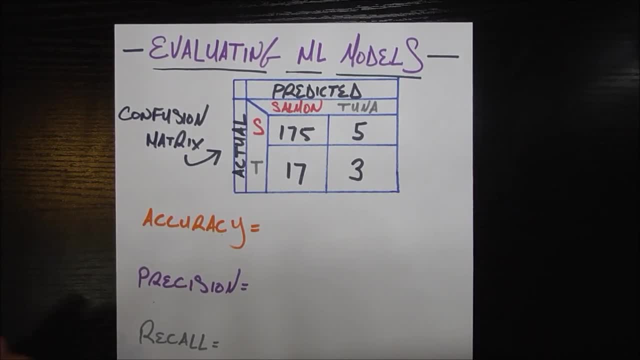 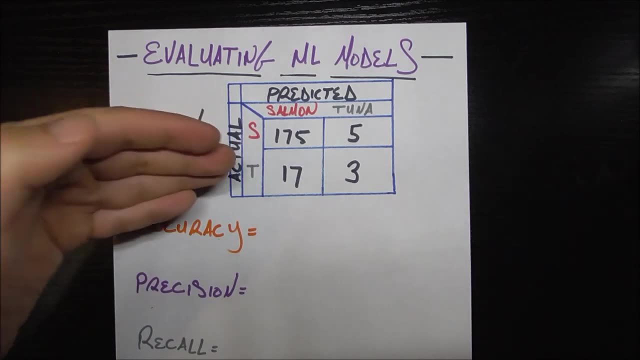 framework we've used in previous videos about we're trying to classify some mystery fish as either a salmon or a tuna, And let's say that we've run whatever machine learning algorithm that we want to run and these are our results. So this type of 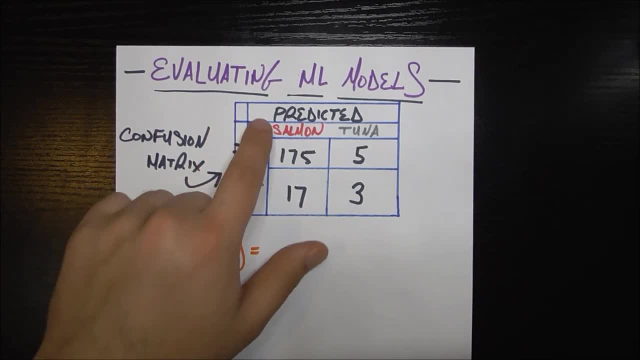 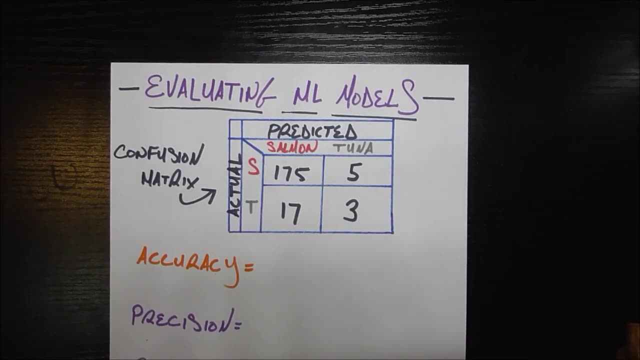 matrix that we're going to be using is called accuracy, And we're going to use this type of matrix right here, where we have our actual labels on the left and we have our predicted labels up here on the top. It's called a confusion matrix And it basically just tells us how many. 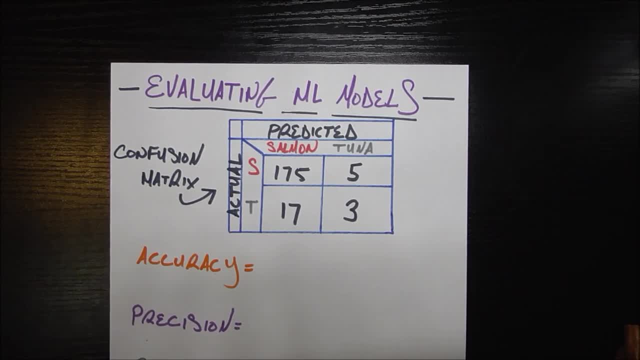 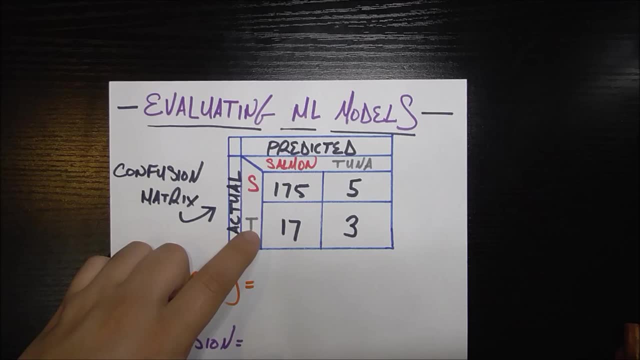 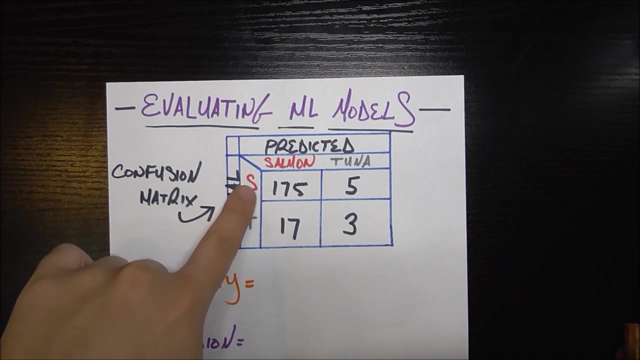 things we got correct out of each category that we predicted. So let's get a little bit familiar with this matrix before looking at the different metrics we'll use. So S is salmon, T is tuna, For example. this 5 right here says that there was five cases where the mystery fish was actually a. 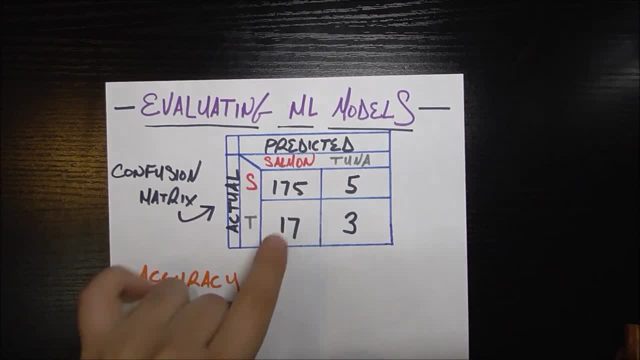 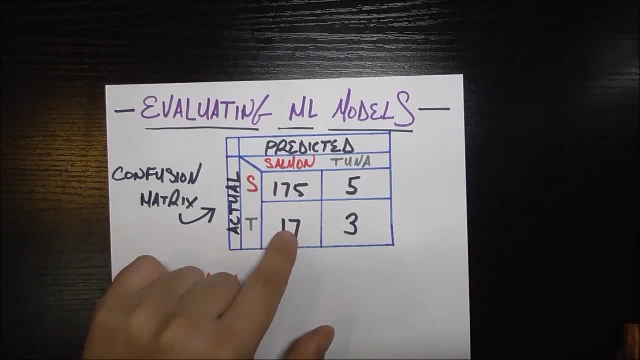 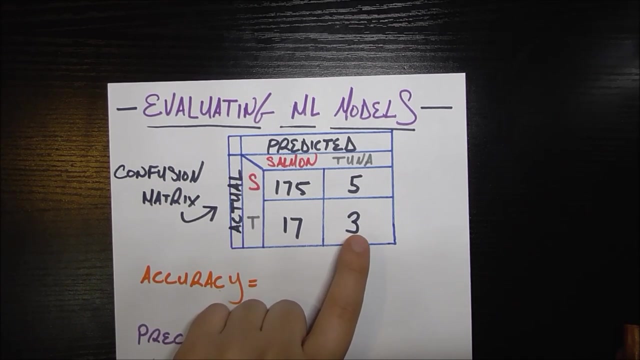 salmon, but I predicted it to be a tuna, So I was wrong here. This is also a wrong situation. It's just the other way, where the mystery fish was actually a tuna, but I predicted it to be a salmon. In opposition, we have this three here, which is a correct guess. We're saying here that 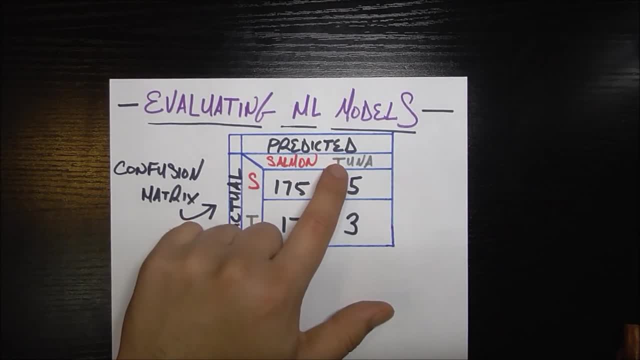 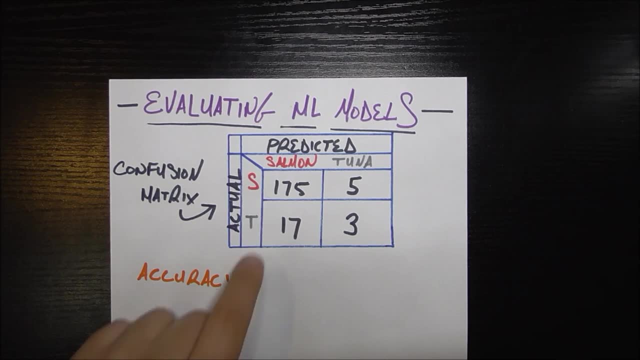 there was three cases where it was actually a tuna and we predicted it to be a tuna, Okay. So one thing to note right here is that we had many, many more salmon than tuna. So we're going to go ahead and calculate the accuracy metric. So we had, it seems, like 180 salmon, 175 plus 5.. 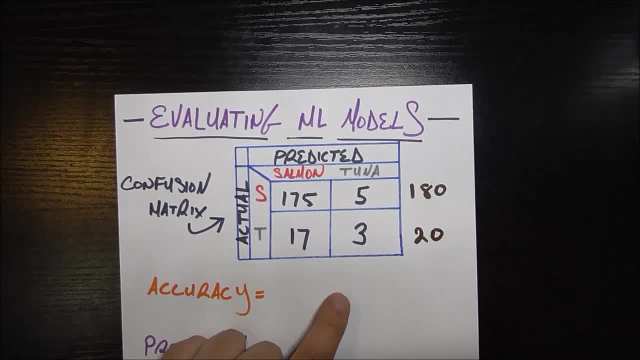 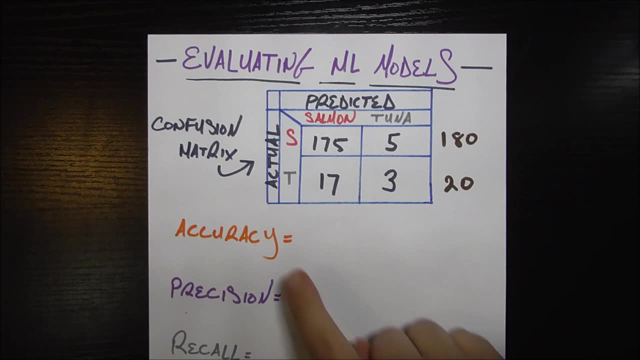 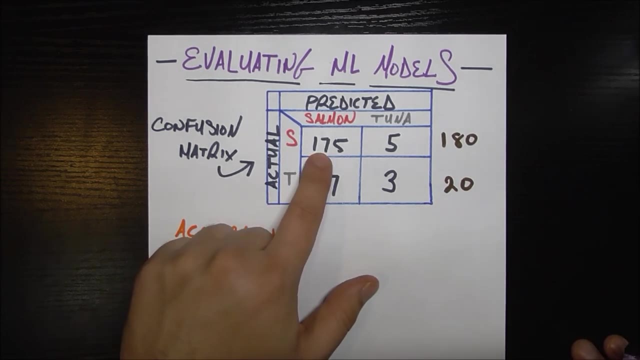 So there's 180 actual salmon and 20 actual tuna. Okay, So let's go ahead and calculate that seemingly obvious accuracy metric, right? So accuracy simply measures how many correct guesses I made out of how many total guesses I made. So correct would be this: 175,, which is 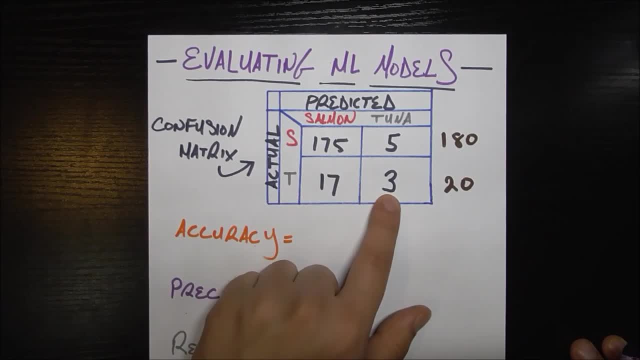 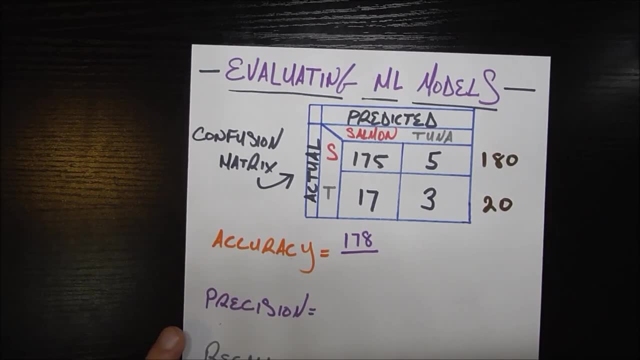 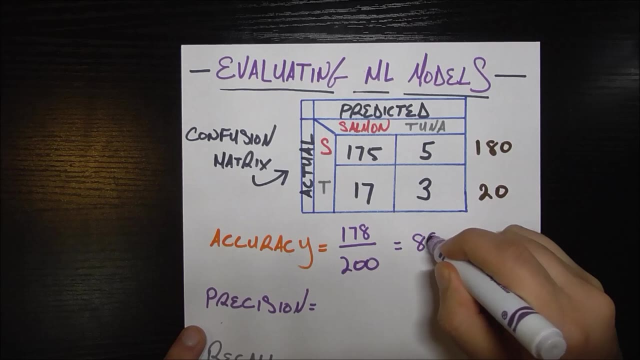 predicting salmon, and it's actually a salmon, plus this three predicting tuna, and it's actually a tuna. So I get 178 correct guesses. Out of how many total guesses? if you add all this up, this 180 and 20, it's 200.. So our accuracy comes out to, it turns out. 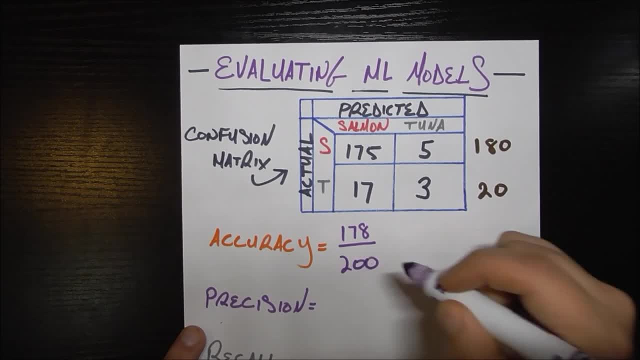 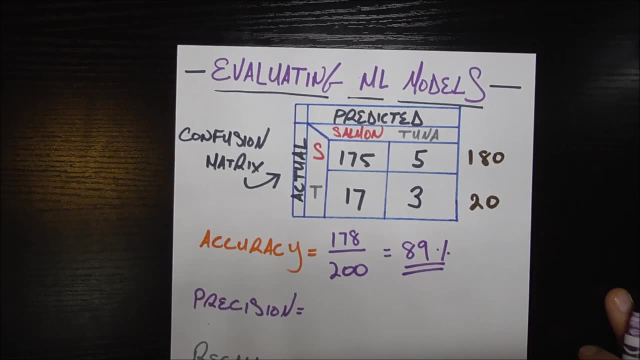 add all this up, this 180 and 20, it's 200.. So our accuracy comes out to: it turns out something like 89%. So it seems pretty good, right, We're getting a really high accuracy. So what's the problem? Well, here's the issue. Let's say that our whole goal here was to correctly 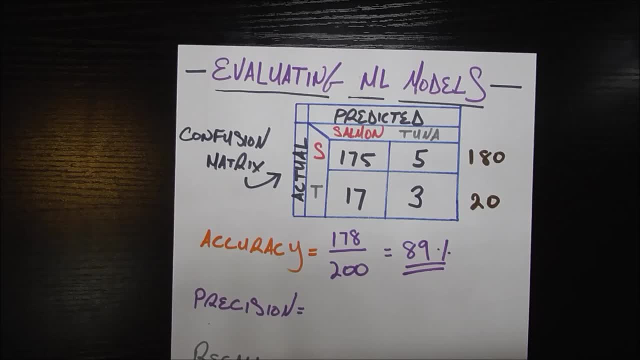 predict tuna because, let's say, in our area they're going extinct and we want to make sure to catch every tuna and not miss any with our prediction algorithm. So let's see if we're doing a good job, if that's our goal. A new metric that we will introduce here is called precision. 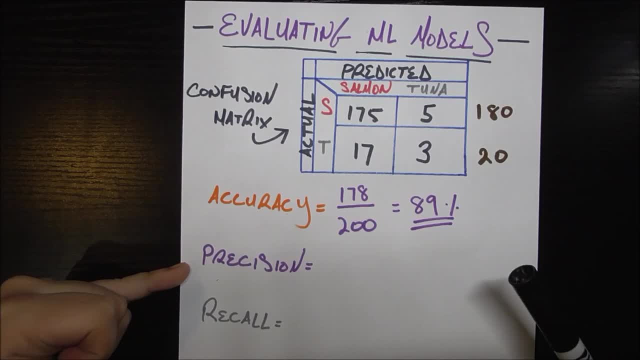 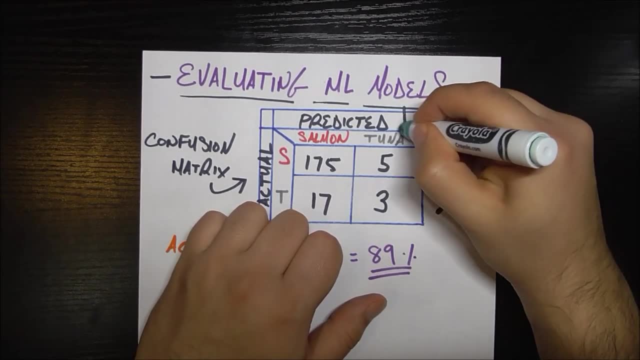 Precision is given by: out of all the guesses you make for your target class, how many did you get correct? So, since our target class here is tuna, we go ahead and look at this column. So we made eight total guesses. We're going to go ahead and look at this column, So we made eight total. 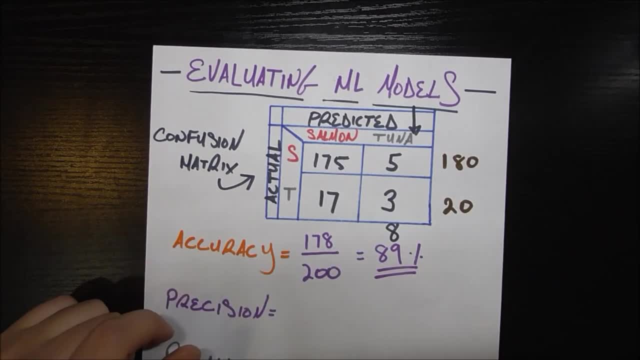 guesses. We're going to go ahead and look at this column. So we made eight total guesses. We're going to go ahead and look at this column. So we made eight total guesses for tuna right, Five and three Out of those eight. how many did we get correct? Only three of them. So our precision: 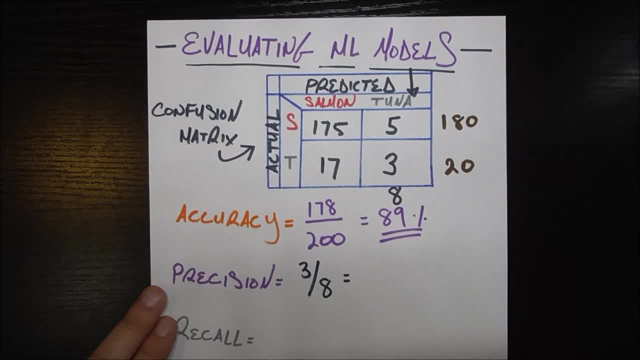 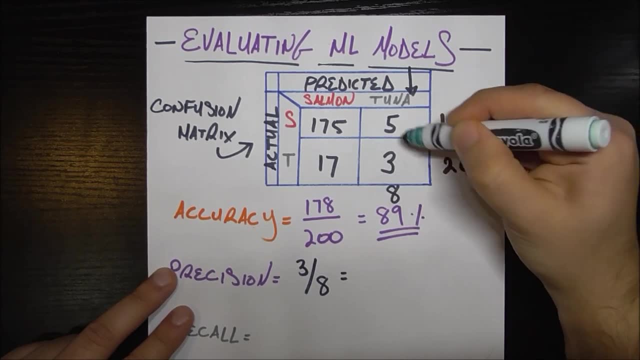 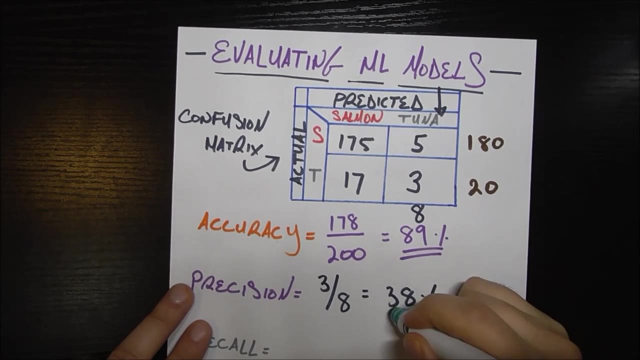 is three out of eight, To just repeat myself, to make sure this sinks in. this precision is out of all the ones where I guessed it was a tuna. how many did I actually get it correct, right on the mark? So three out of eight, that comes out to about 38%, right, So not looking as good as that. 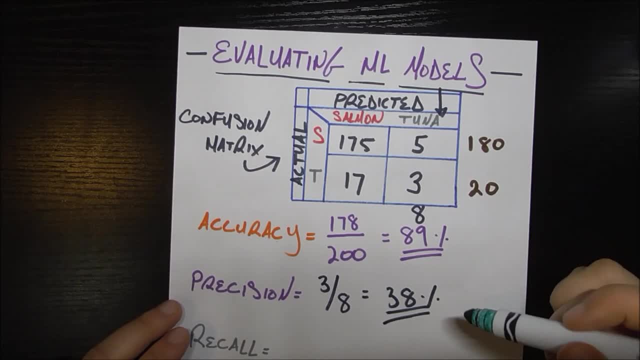 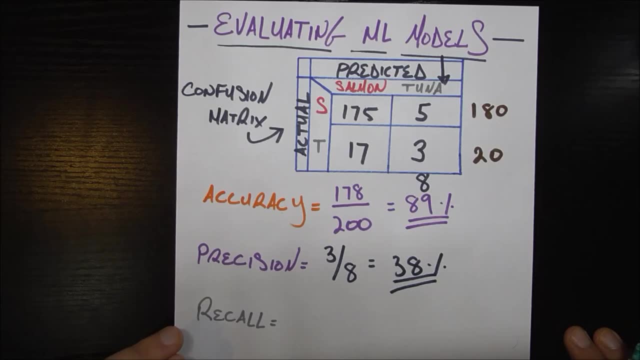 89% anymore. Really not looking very good at all. So we're going to go ahead and look at this column to see if we get at all. Now let's look at a different metric, also called recall Recall measures, a slightly different thing with a different notion. Recall measures, out of all the things that were. 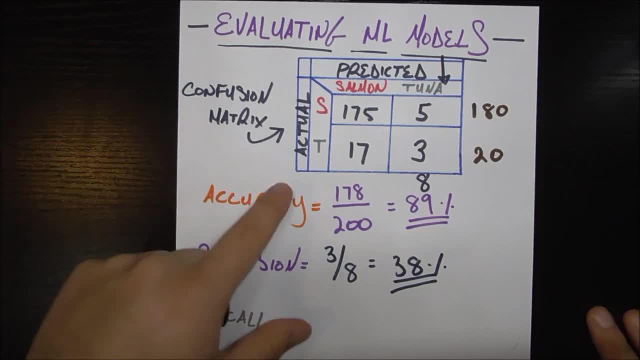 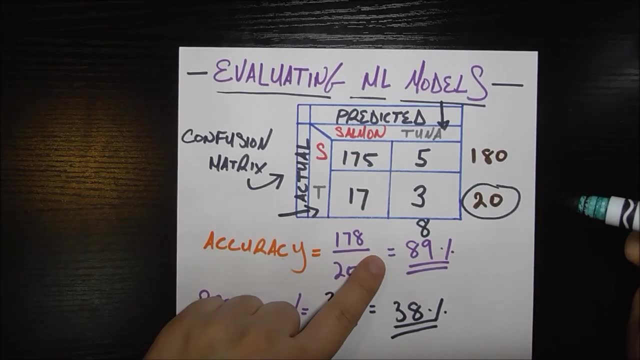 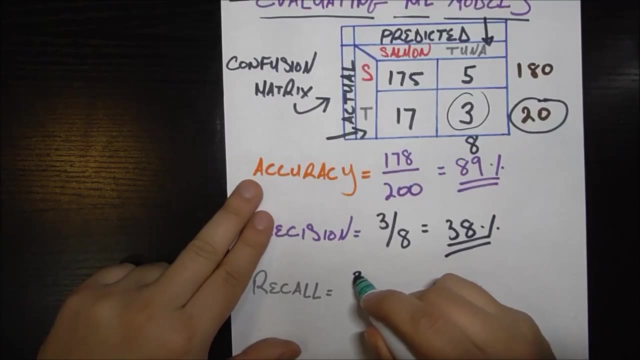 actually tuna. how many did I catch as tuna? So that's subtly different, because now we're looking at this row of things actually being tuna. So out of these 20 fish that were actually tuna, how many did I correctly classify as tuna? It turns out I got only three of them, So that would 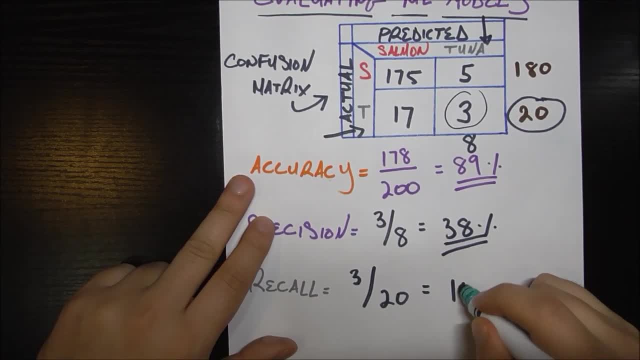 be three out of eight. So that's a little bit of a difference. So we're going to go ahead. and three out of 20, which is a measly 15%. So our recall is very, very, very low. Our precision. 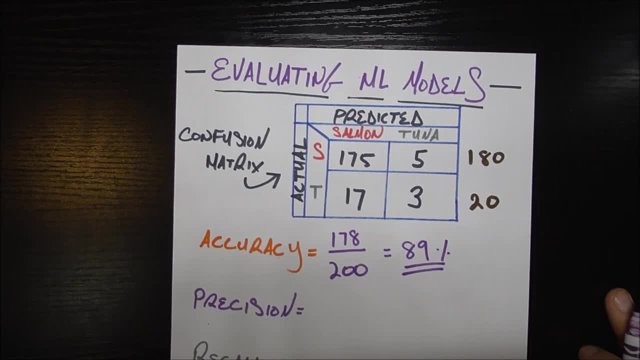 something like 89%. So it seems pretty good, right? We're getting a really high accuracy. So what's the problem? Well, here's the issue. Let's say that our whole goal here was to correctly predict tuna because, let's say, in our area they're going extinct and we're 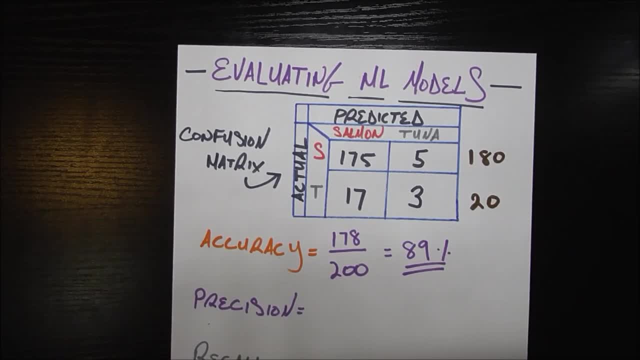 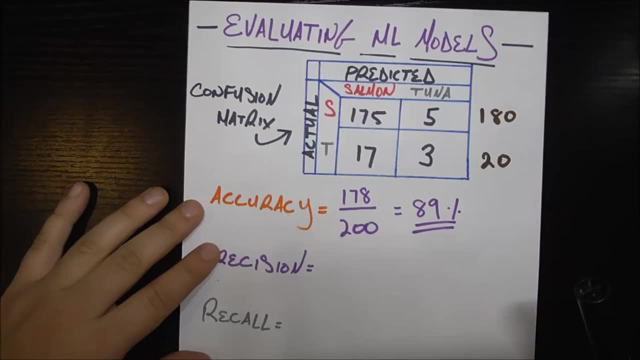 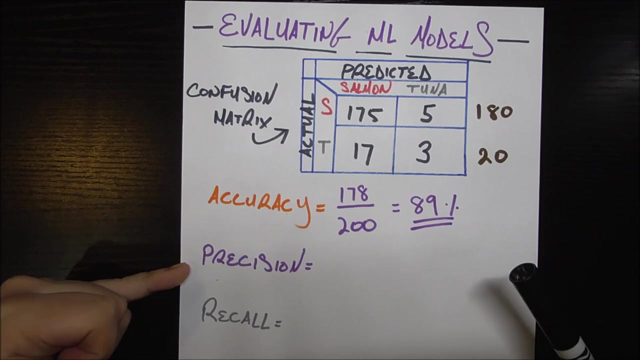 going to have to catch every tuna and not miss any with our prediction algorithm, So let's see if we're doing a good job, if that's our goal. A new metric that we will introduce here is called precision. Precision is given by out of all the guesses you make for your target class. 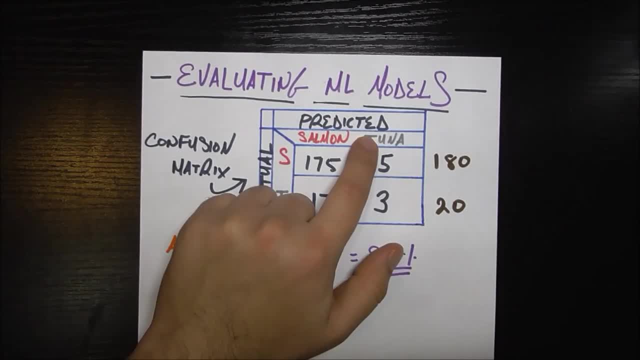 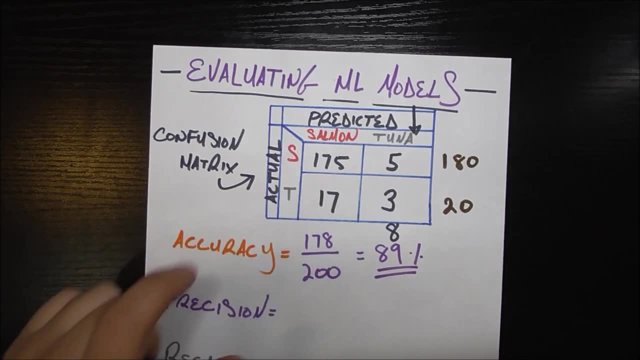 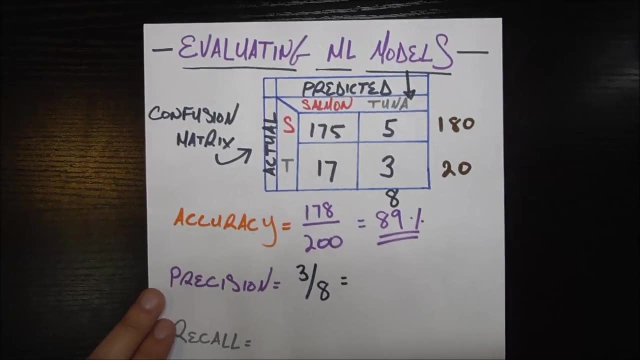 how many did you get correct? So since our target class here is tuna, we go ahead and look at this column. So we made eight total guesses for tuna right: Five and three Out of those eight. how many did you get correct? Only three of them. So our precision is three out of eight, To just 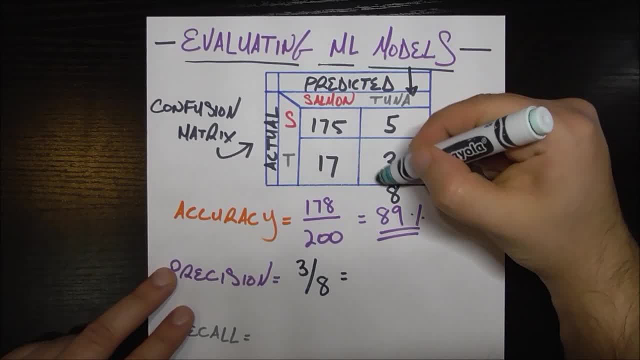 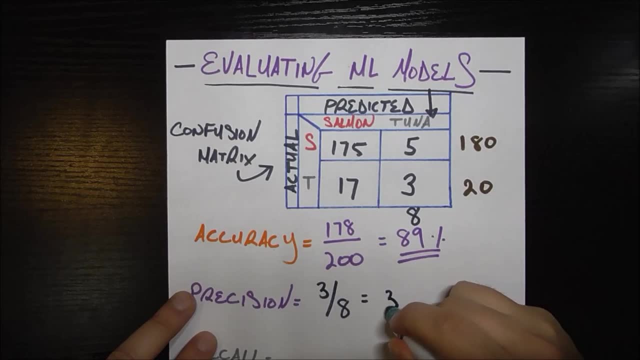 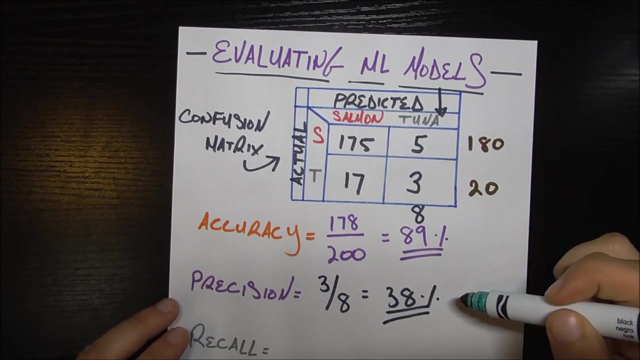 repeat myself to make sure this sinks in. this precision is out of all the ones where I guessed it was a tuna, how many did I actually get it correct, right on the mark. So three out of eight. that comes out to about 38%, right? So not looking as good as that 89 anymore. really not looking. 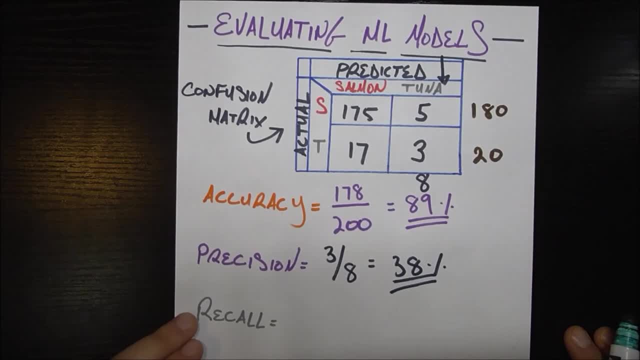 very good at all. Now let's look at a different metric, also called recall, Recall measures, a slightly different thing with a different notion. Recall measures: out of all the things that were actually tuna, how many did I catch as tuna? So 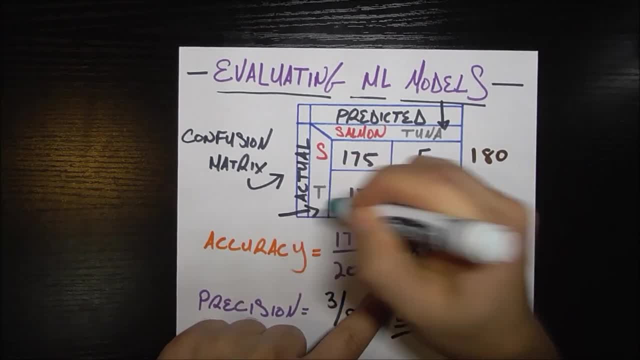 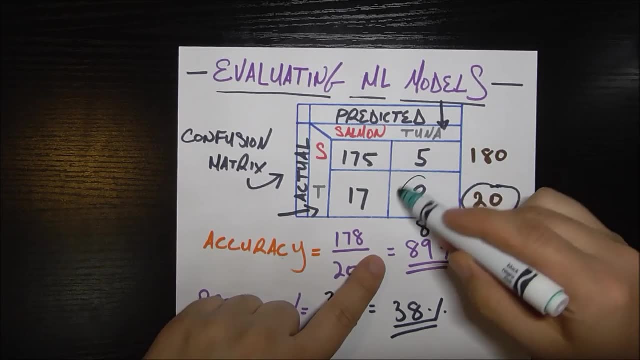 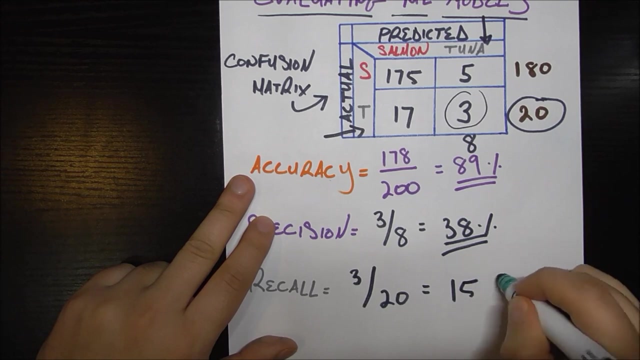 that's subtly different, because now we're looking at this row of things actually being tuna. So out of these 20 fish that were actually tuna, how many did I correctly classify as tuna? It turns out I got only three of them, So that would be three out of 20, which is a measly 50%. 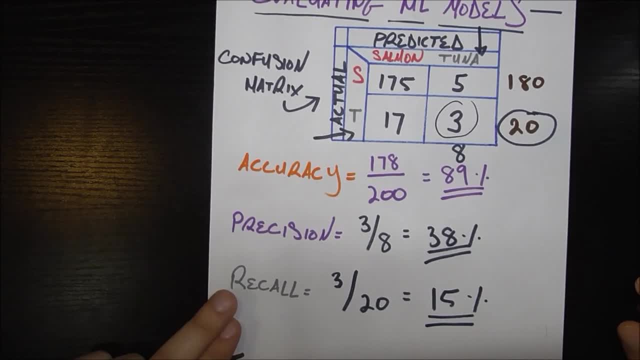 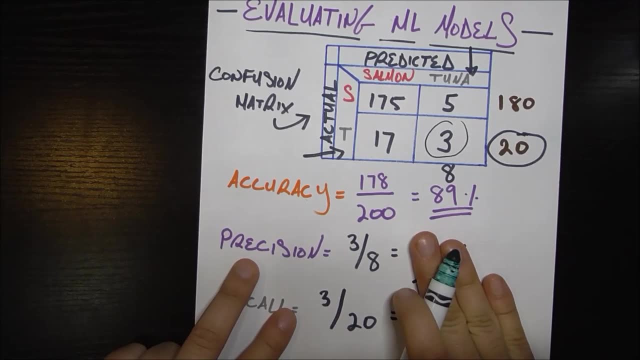 of the total. So that's a pretty good estimate. And then we look at the accuracy, which is 15%. So our recall is very, very, very low. Our precision is also rather low, but our accuracy is high. So we wouldn't looking at accuracy by itself. we wouldn't know the full. 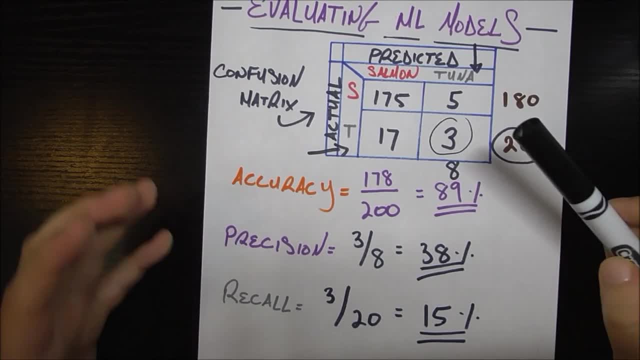 story. We need to look at precision and recall as well to see how good of a job we're doing. Now you might be asking: oh, there's so many metrics, how do I know which one to use? Well, the answer is: it depends. It depends on what's your goal. 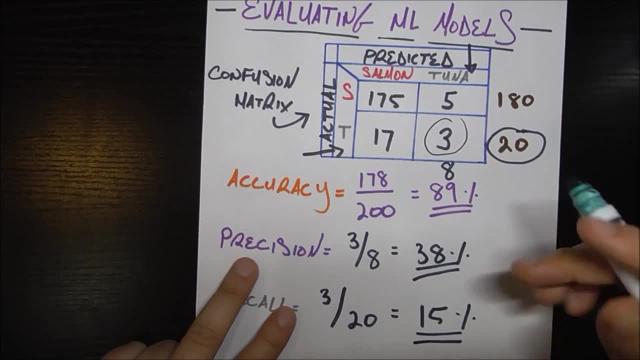 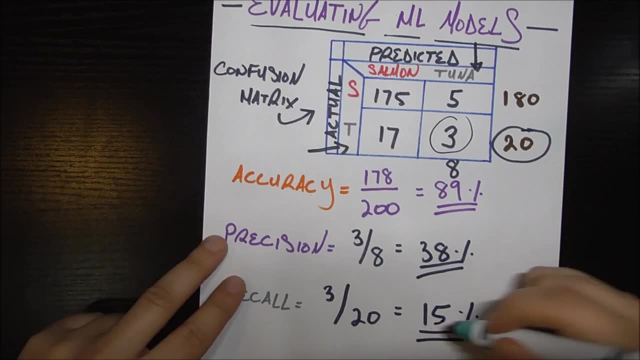 is also rather low, but our accuracy is high. So we wouldn't. we wouldn't looking at accuracy by itself, we wouldn't know the full story. We need to look at precision and recall as well to see how good of a job we're doing. Now you might be asking: oh, there's so many metrics, How do I? 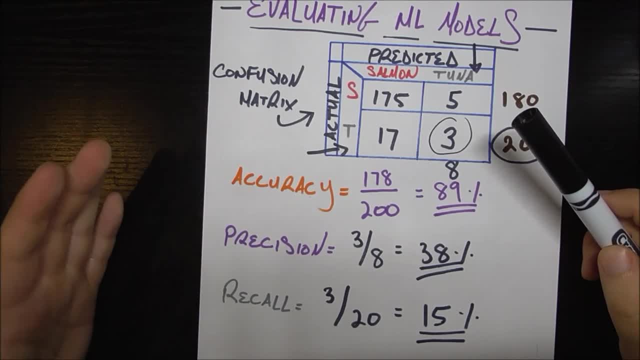 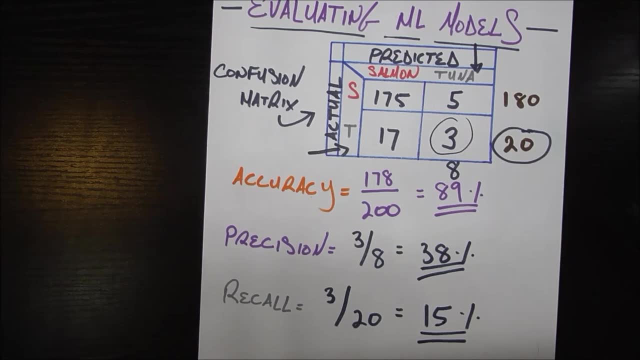 know which one to use. Well, the answer is it depends. It depends on what's your goal. If you have different goals, different of these metrics are going to be important. Just to give a quick introduction to a couple real life scenarios. If you're trying to for 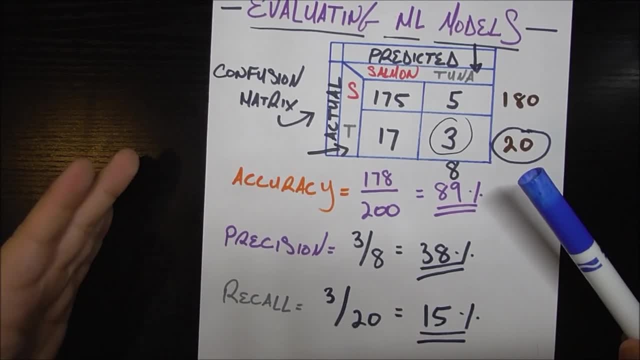 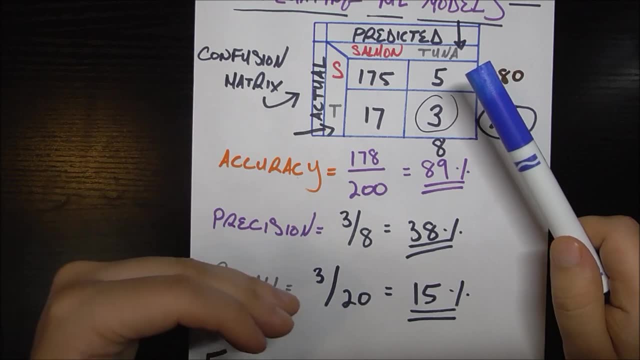 example, predict students at risk of dropping out of your college or your high school or something you probably really care about. recall, because you care about. of all the students that are going to drop out, I want to make sure that I catch a very high percentage of them. 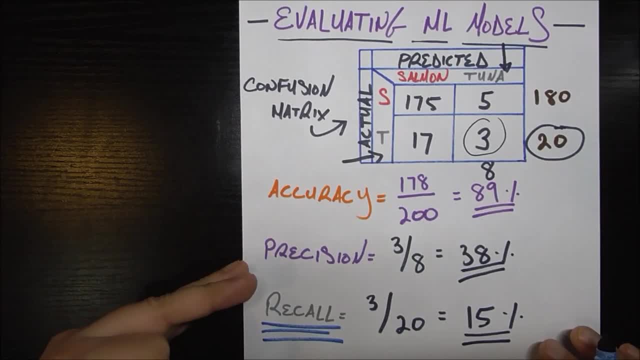 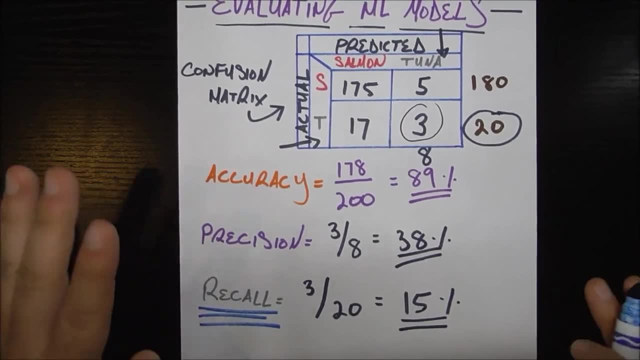 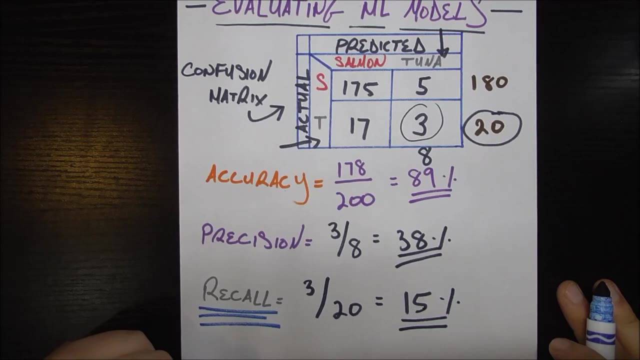 Which means that I want a very, very high recall. It's okay if my precision is not so high in that case, because if my precision is low I potentially catch a bunch of students who weren't going to drop out, but it doesn't really hurt me to try to give them resources either way. Now a case where 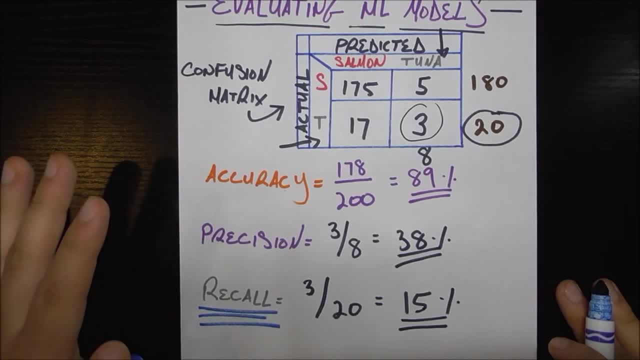 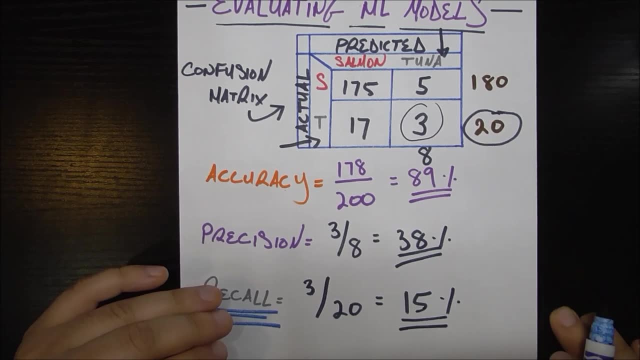 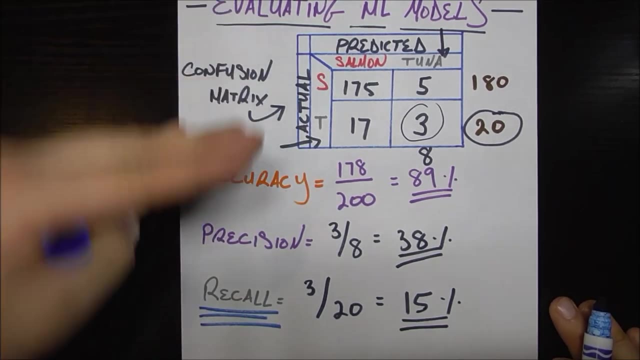 precision might be. more important is, if I'm trying to select students at my school to represent the whole school in some national competition, I want to make sure that whatever method I'm using, I'm using to pick students who are very qualified to represent the school. I'm picking only qualified. 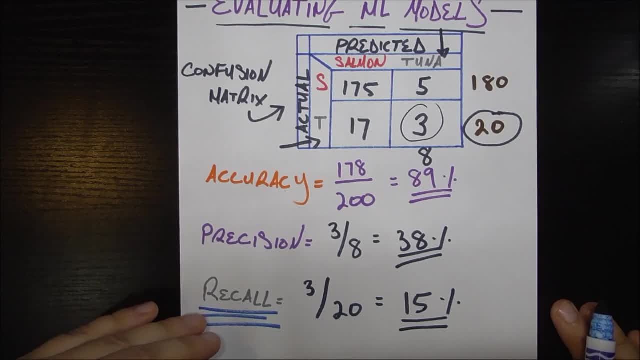 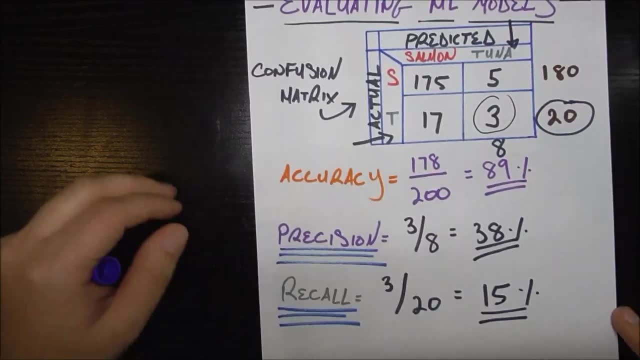 students. It's okay if my recall is not that high, which means that I'm not picking all qualified students. I just care that of all the students I pick, a big percentage of them- a big precision- are qualified to represent the school. So those are just two cases where precision might be more. 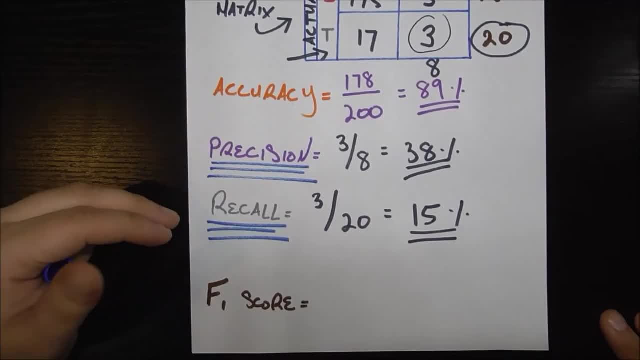 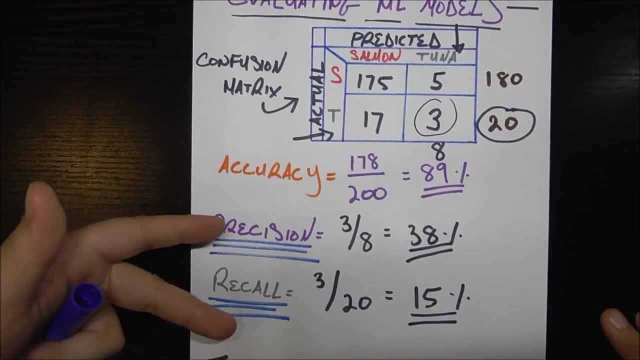 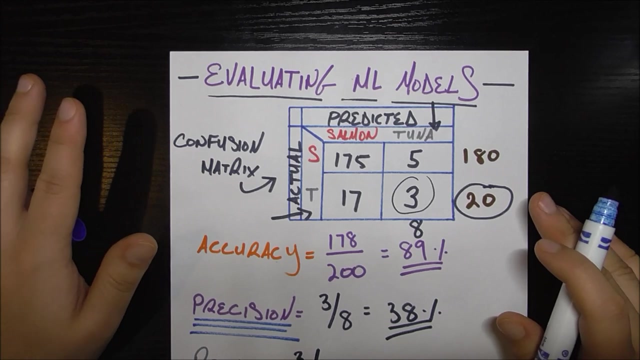 important, or recall might be more important. Of course, they both are pretty important. So how do we combine both Both of them? And before I go into what the F1 score is, there's a way to game both of these metrics. For example, I can make a recall 100% if I just classify everything as a tuna, So all I do is 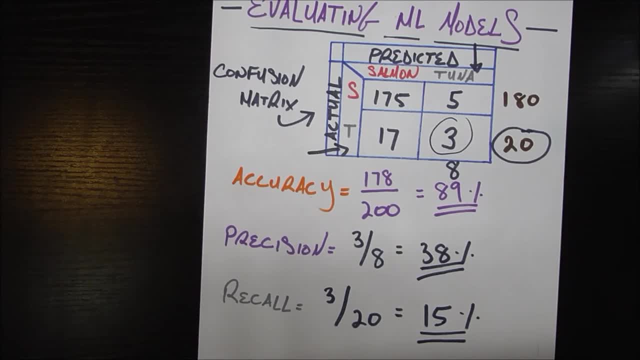 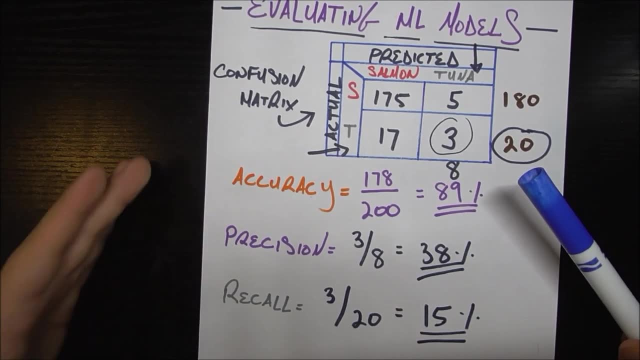 If you're trying to, for example, predict students at risk of dropping out of your college or your high school or something you probably really care about. recall, because you care about of all the students that are going to drop out. I want to make sure that I catch. 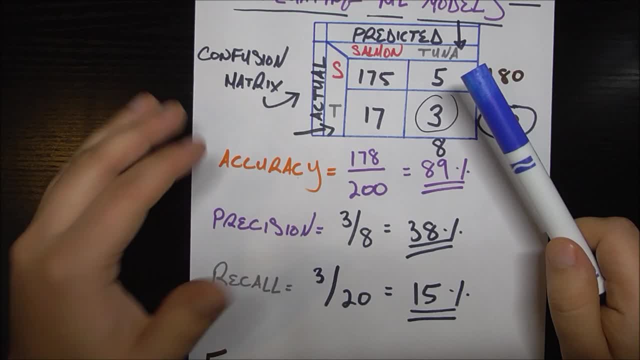 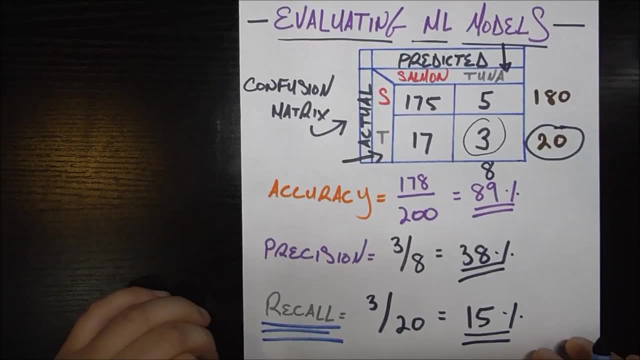 a very high percentage of them, which means that I want a very, very high recall. It's okay if my precision is not so high in that case, because if my precision is low, I'm going to be able to catch a very high percentage of them. So I'm going to be able to catch a very high percentage of them. 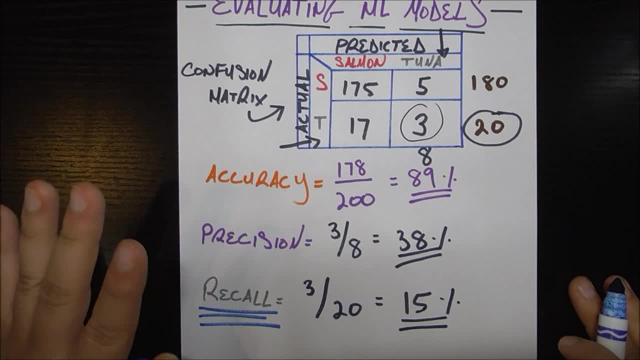 I potentially catch a bunch of students who weren't going to drop out, but it doesn't really hurt me to try to give them resources either way. Now, a case where precision might be more important is if I'm trying to select students at my school to represent the whole school in. 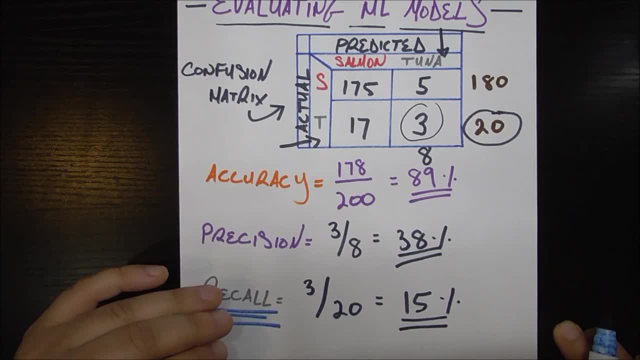 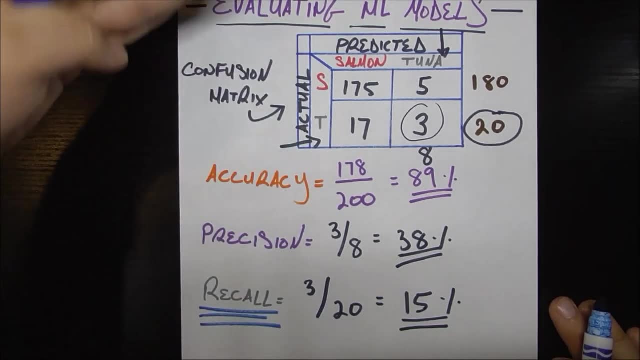 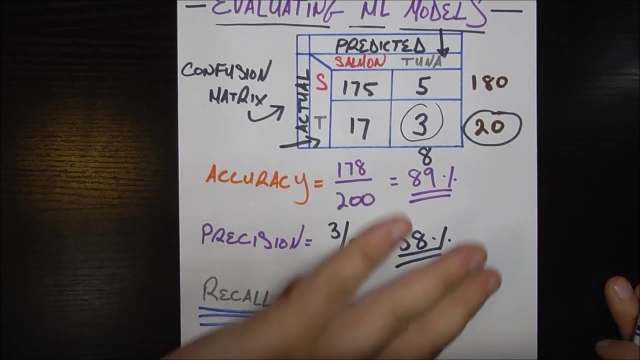 some national competition. I want to make sure that, whatever method I'm using to pick students who are very qualified to represent the school, I'm picking only qualified students. It's okay if recall is not that high, which means that I'm not picking all qualified students. I just care that. 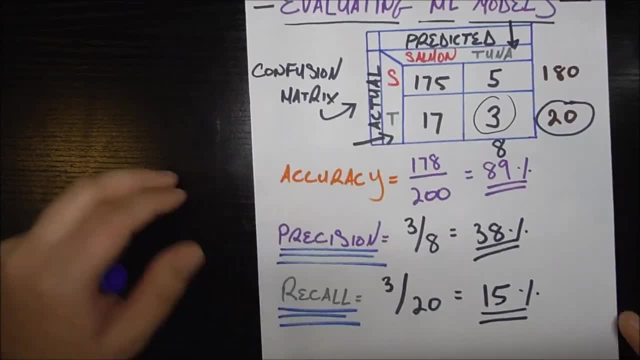 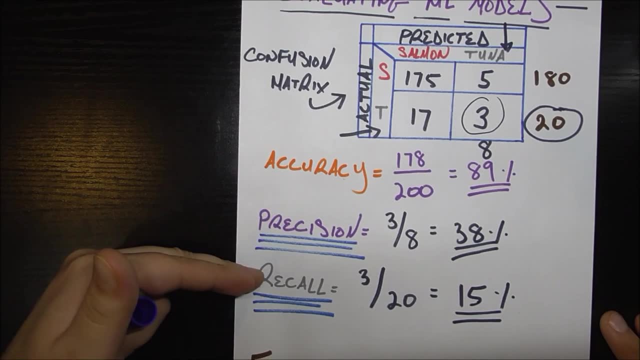 of all the students I pick. a big percentage of them, a big precision are qualified to represent the school. So those are just two cases where precision might be more important or recall might be more important. Of course, they both are pretty important. So how do we combine both of them? And 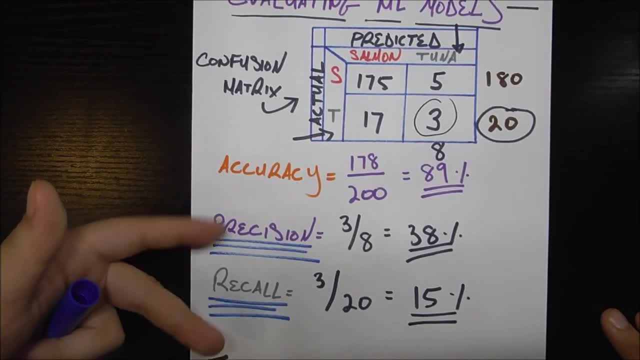 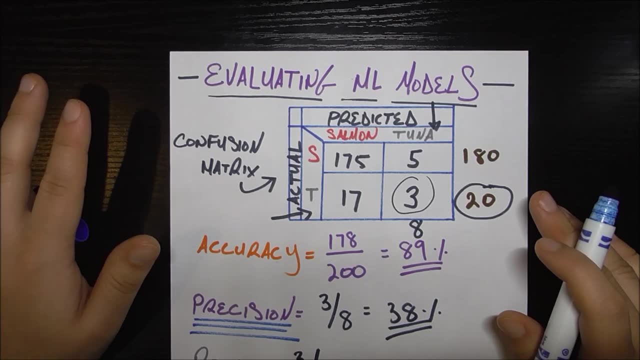 before I go into what the F1 score is, there's a way to game both of these metrics. For example, I can make a recall a hundred percent if I just classify everything as a tuna. So all I do is, every time a mystery fish comes, I say: 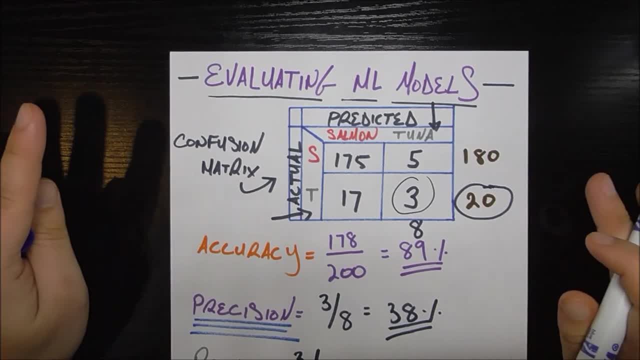 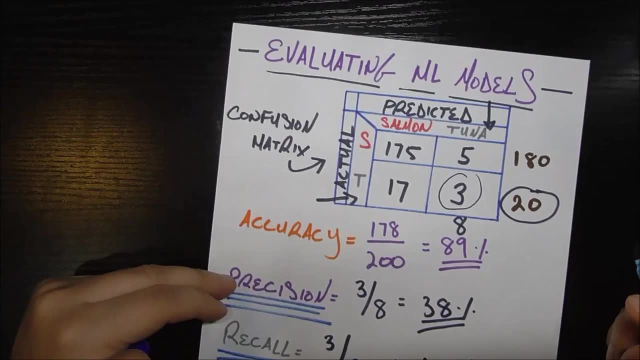 tuna, tuna, tuna. That means that I'm going to catch all the tuna, because I definitely classified everything as a tuna, So my recall will be a hundred percent. My precision probably is going to suck because I classified a bunch of things as a tuna that were not a tuna at all. 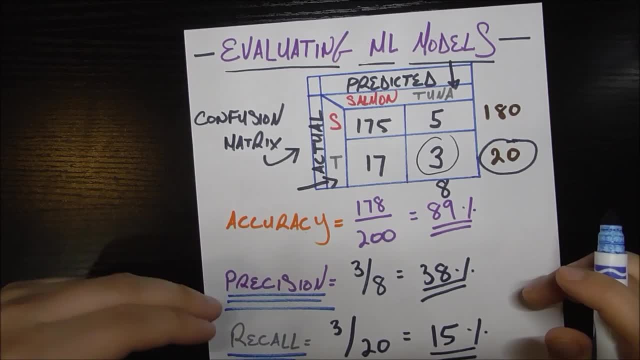 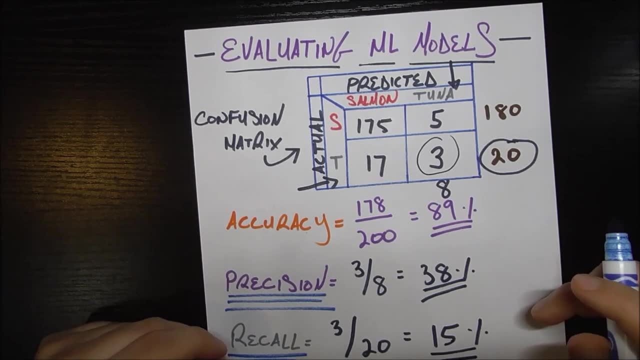 A way to game the precision metric would be, basically: if you only classify something as a tuna, you're going to have a very high precision because you're not really sure. if you're, like, almost a hundred percent sure, In that case you're going to have a very high precision because you don't.